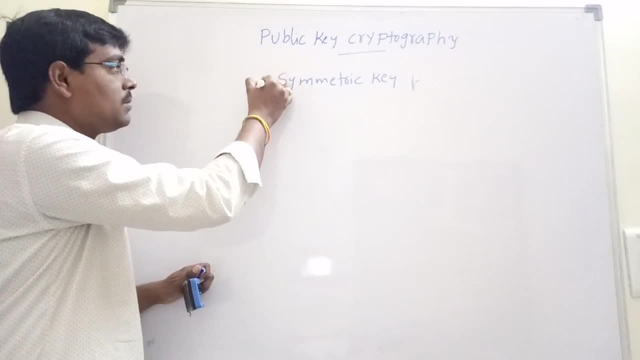 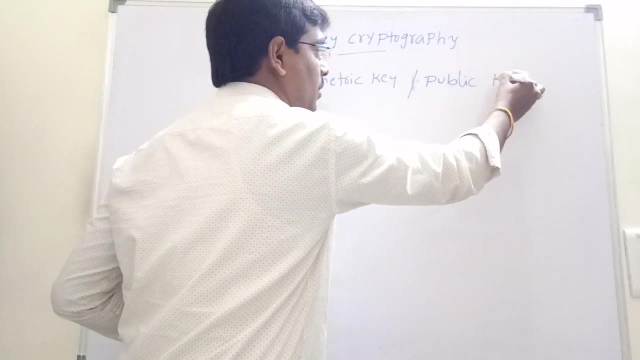 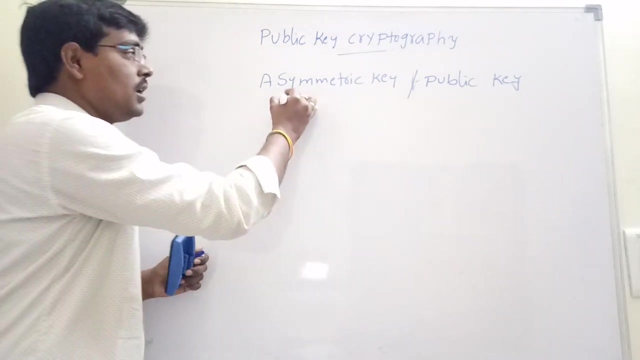 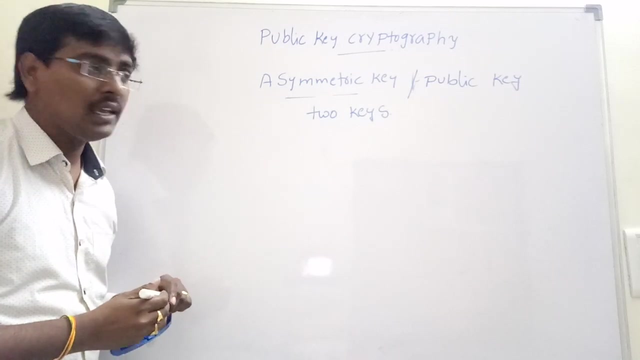 problem. we are moving to some another technique. that is simply asymmetric key cryptography or cryptography, Public key cryptography. So in symmetric, the main problem is: only one key is used for both encryption and decryption. Here we are using two keys. We are using two keys: one key is used for encryption and some other key is used for decryption. 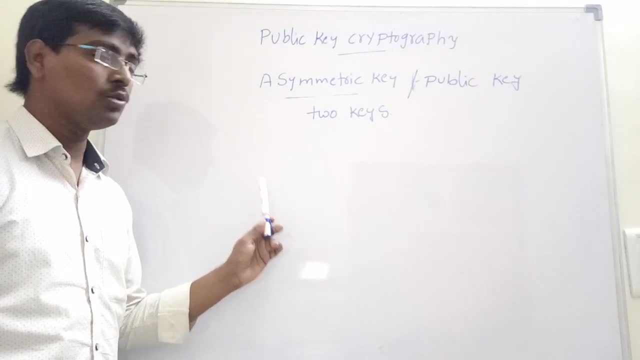 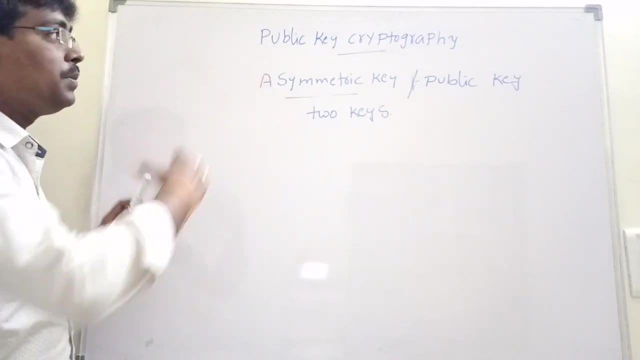 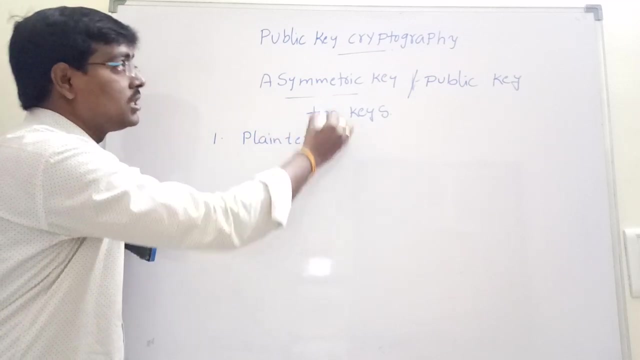 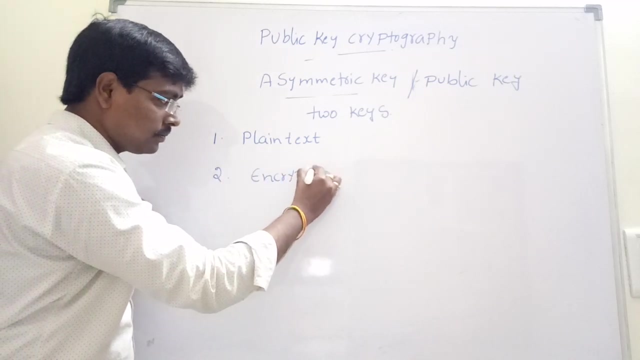 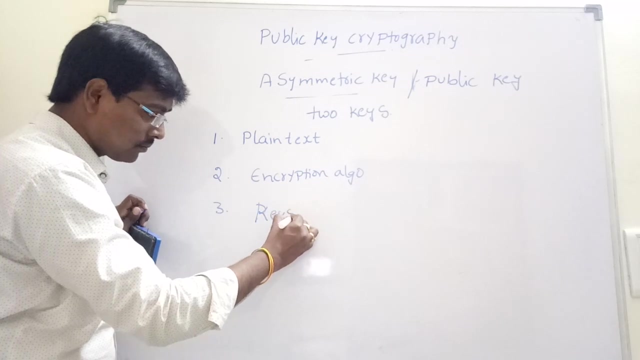 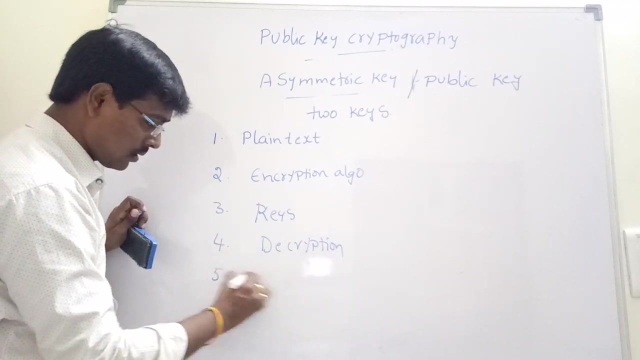 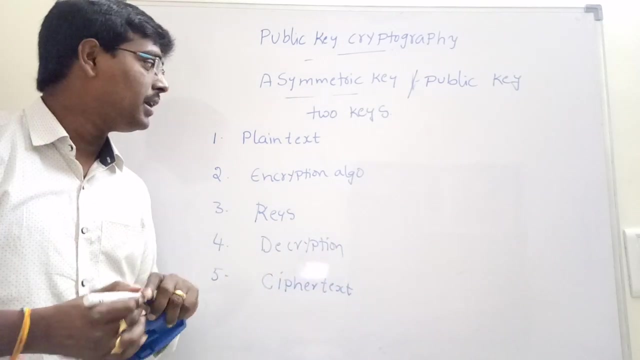 That is, sender performs encrypted operation using one key, Receiver performs decryption operation using some other key. simply, in property cryptography, the elements are plain text. that is this cryptography. what are the elements we have to consider? plain text: encryption algorithm. pop keys, decryption algorithm. encryption algorithm- cipher test. 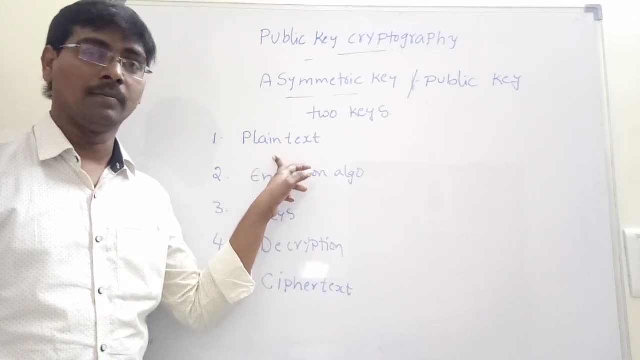 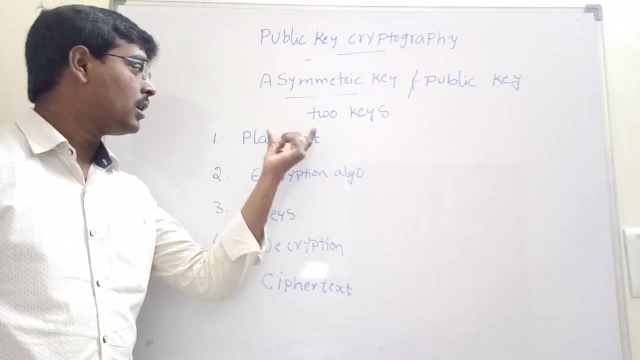 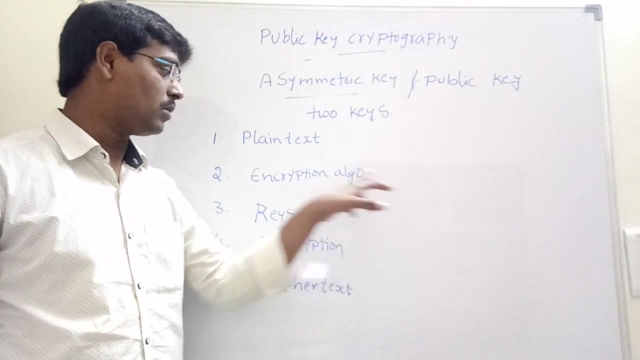 so plain test. plain test is the original message that we want to send. simply, this is an input to the algorithm, that is, the sender wants to send some message, that some message is called plain text encryption algorithm, the plain text is converted into some unreadable format and that 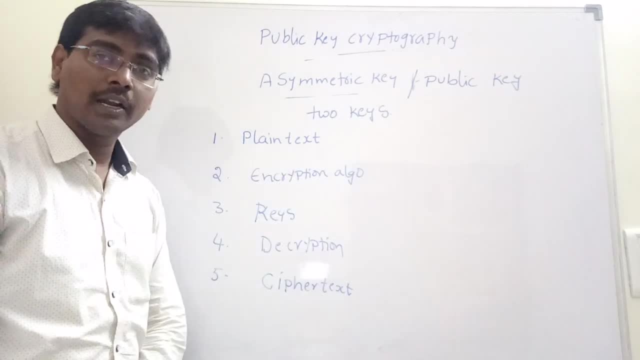 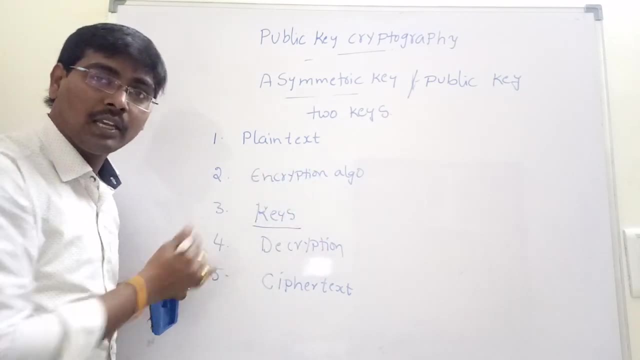 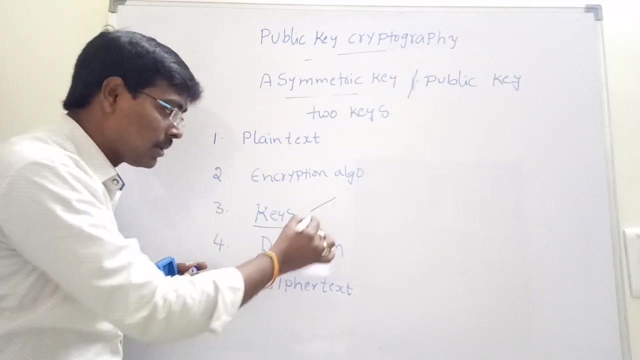 format is sent to the receiver converts the plain test into some unreadable format. that is encryption algorithm keys, here the keys specifies to perform encryption algorithm. we are using some keys generally in asymmetric key cryptography, that is, public key. cryptography keys are divided into two types. one is public key. 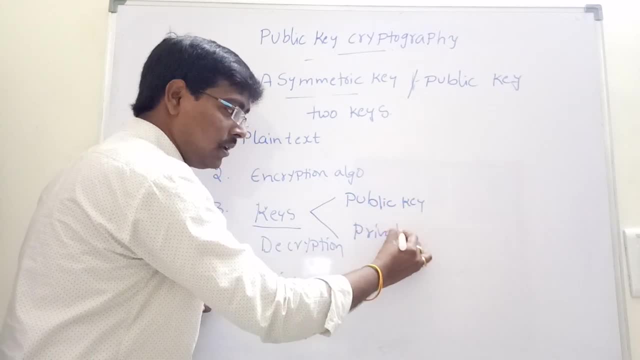 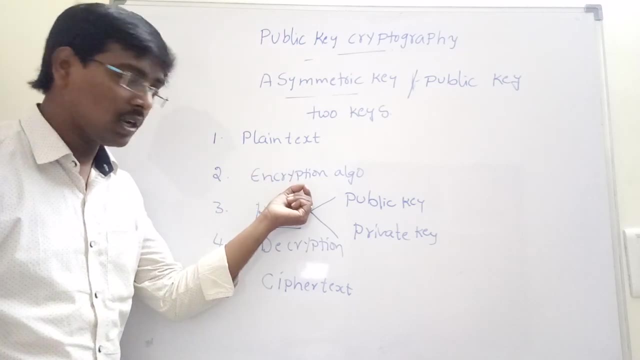 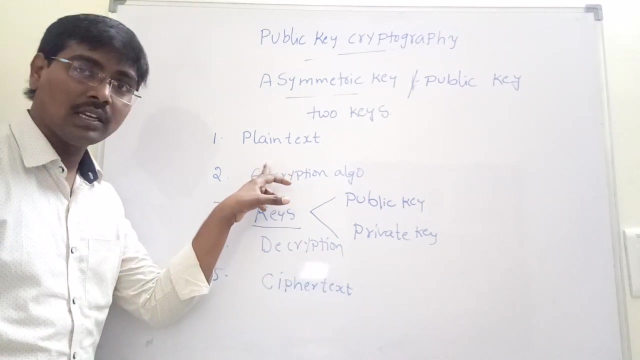 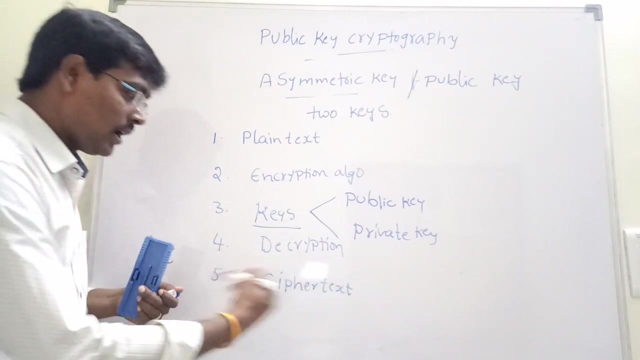 second one is private key, one is public key. second one is private key to perform either encryption operation or decryption. we are using these two key. decryption algorithm means whenever sender send the message to the receiver, that receiver decrypt the message into readable format, and ram test means simply the unreadable message. 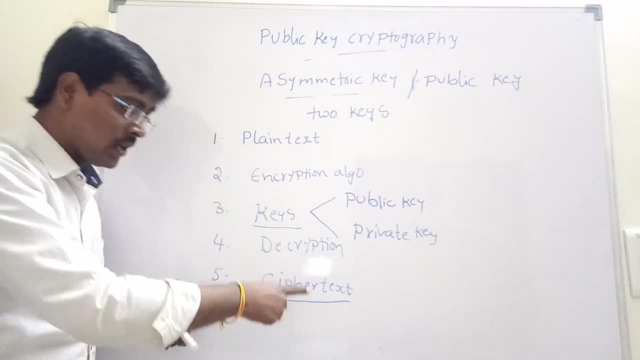 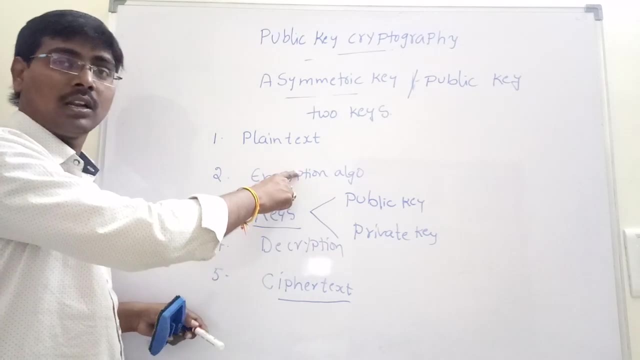 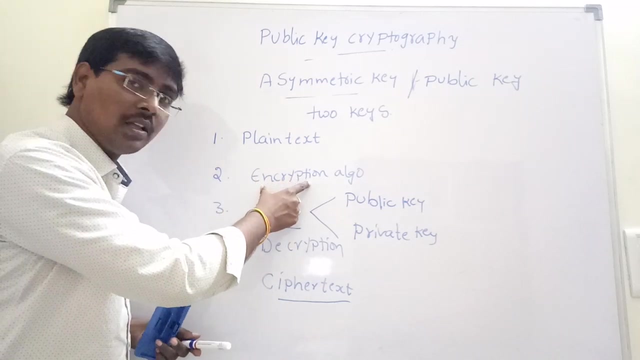 This is So here. Plain test means input to the algorithm. Cipher test means outputting the algorithm To convert plain test into cipher test. we are using some encryption algorithm To convert cipher test into plain test. we are performing some decryption algorithm To perform either encryption algorithm or decryption algorithm. we are using keys. 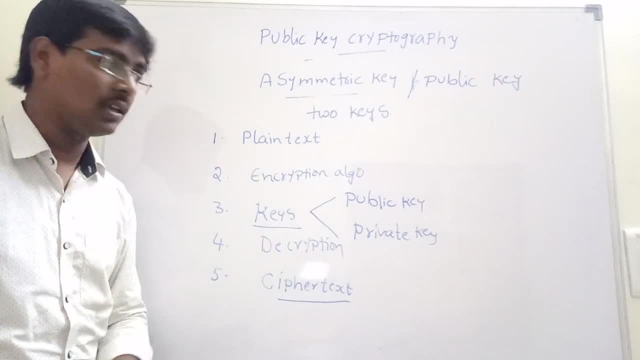 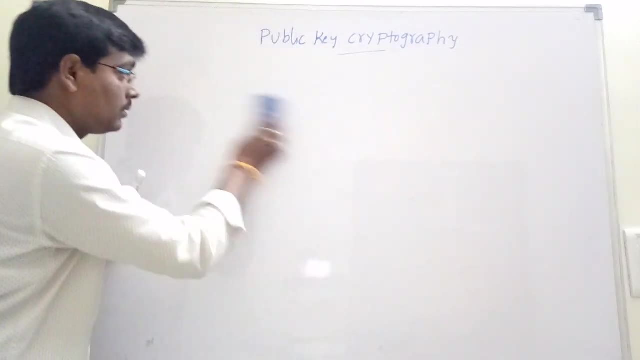 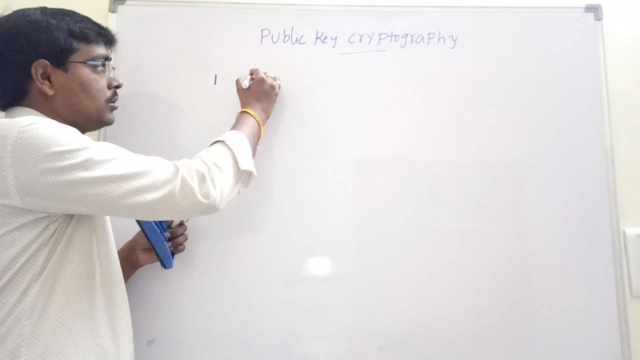 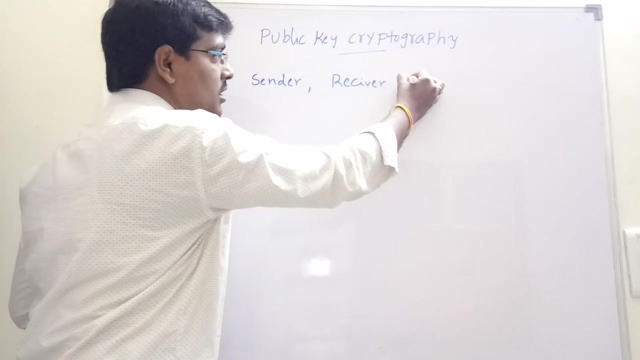 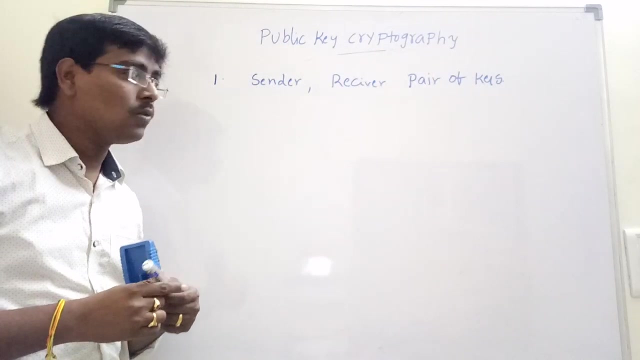 Here in this asymmetric, we are using public key and private key. Now we will discuss public key and private key. The procedure for sending messages to the receiver are: First, both sender and receiver generates a pair of keys, Suppose if a sender wants to send some message to receiver B. 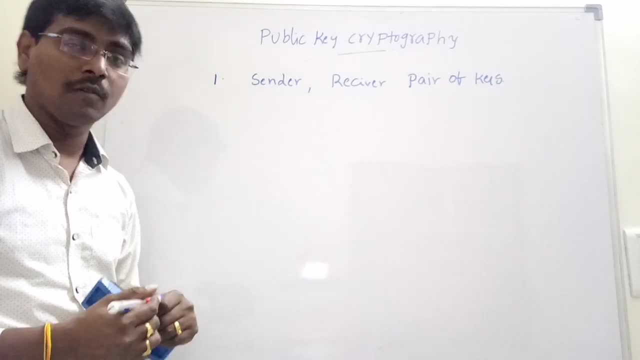 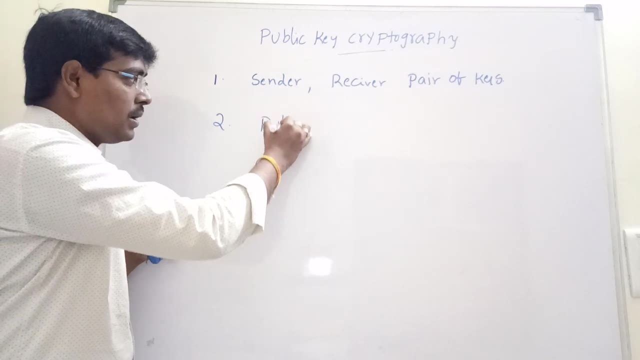 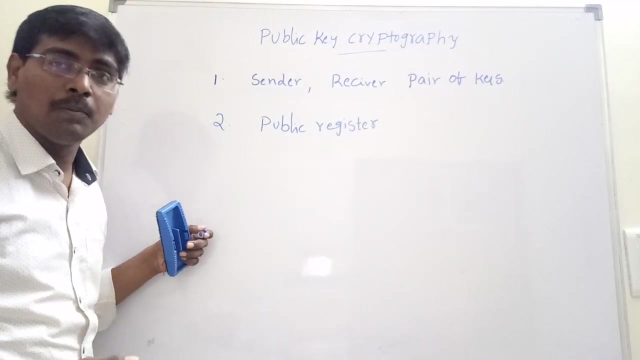 both sender and receiver generates a pair of keys. So pair means two keys In the pair of keys. one key is placed in public register. Among these two keys, one key is placed in public register. That means the key acts as public key. 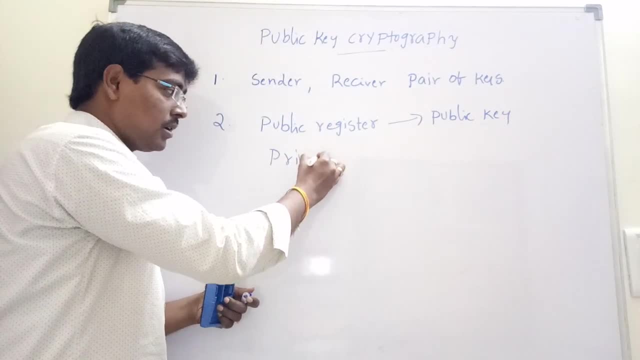 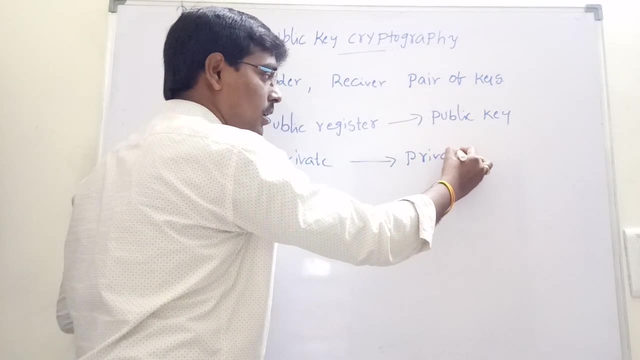 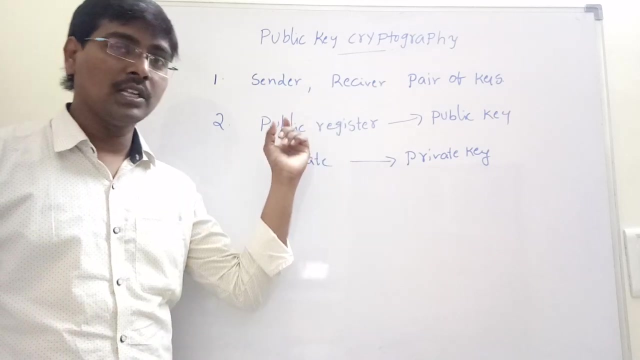 And one key is kept as private. One key is kept as secret. That key is called private key. That key is called private key. That is, each user generates a pair of key. One key is placed in public register. That means that key is visible to all other users in a system. 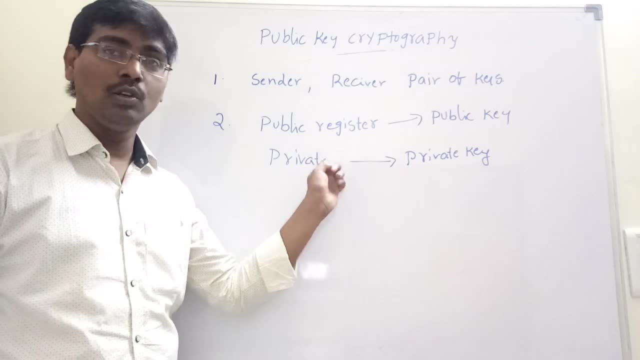 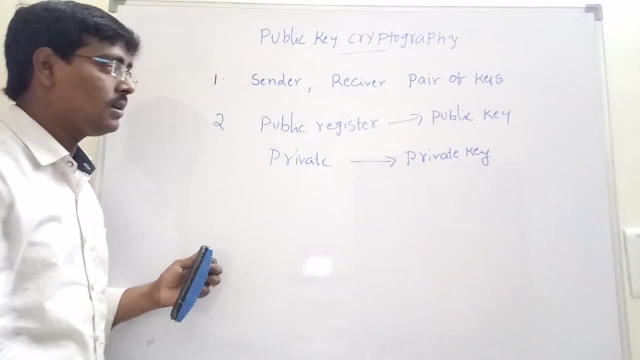 And one key is kept as secret, That is, that is visible to only the user who generates the key In. the key placed in public register is called public key. The key what were kept as secret is called private key. Once this is kept as secret, the key is called private key. 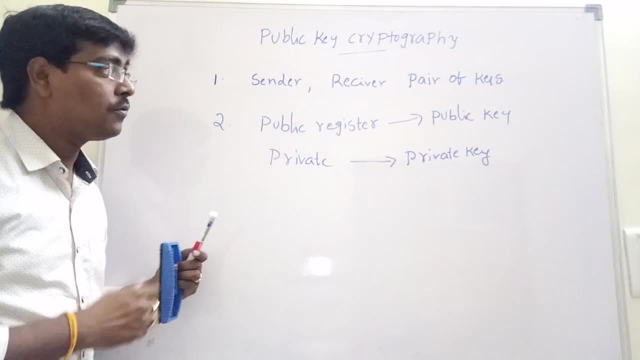 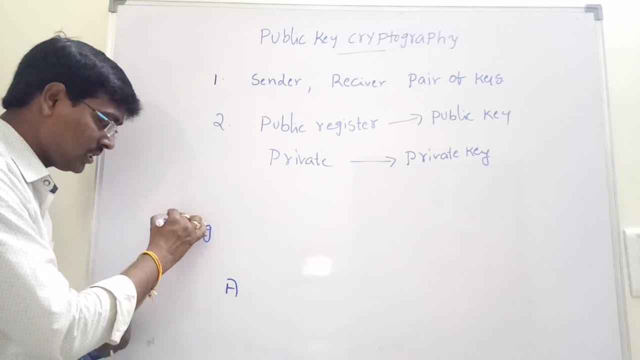 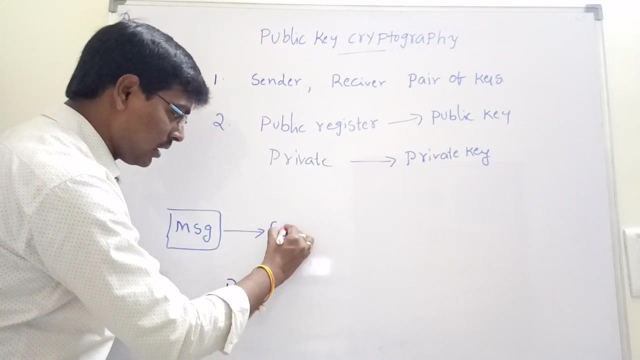 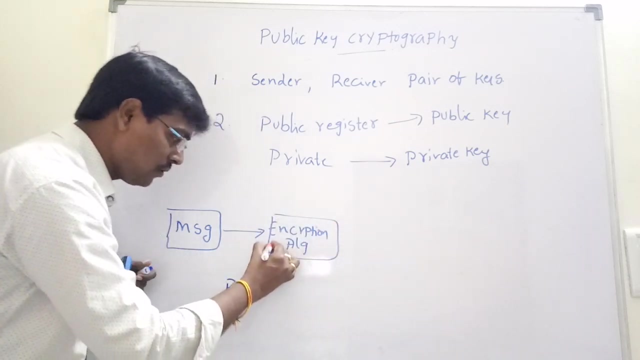 Once these two keys are generated, we are performing encryption and decryption operation. For example, user A wants to send some message. User A wants to send some message. First it performs some encryption operation, Suppose some encryption algorithm, Suppose if the message is X. 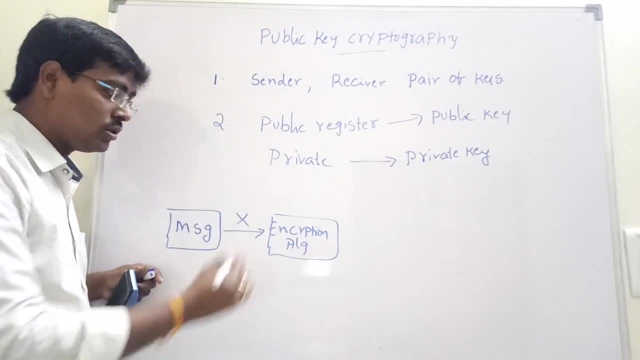 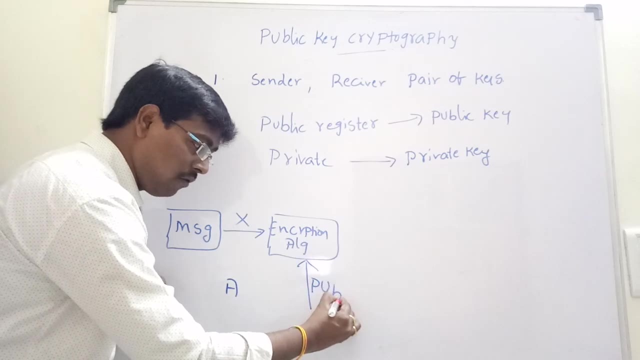 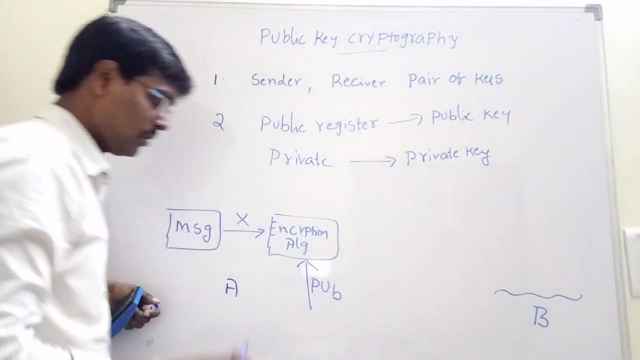 To perform this encryption algorithm we are using some key. For example, if we are using the public key of B, Suppose user A wants to send some message to user B- Send message to user B. We have two types of encryptions and decryptions. 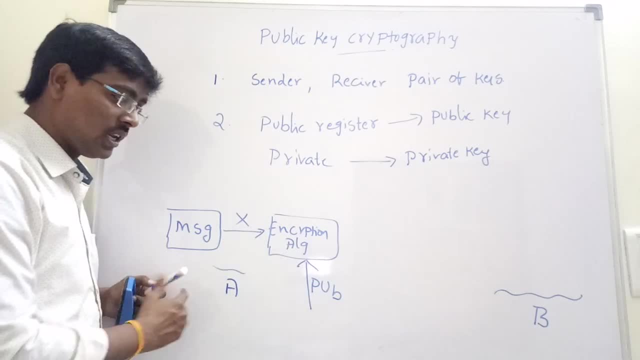 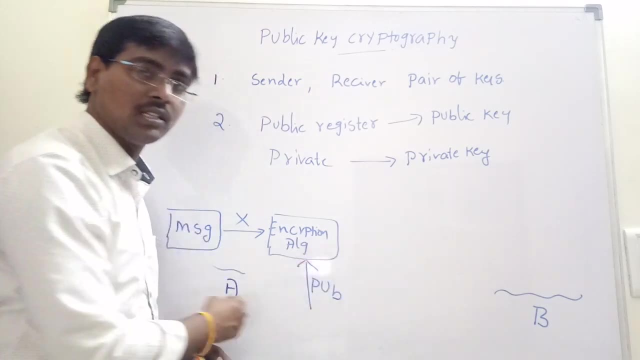 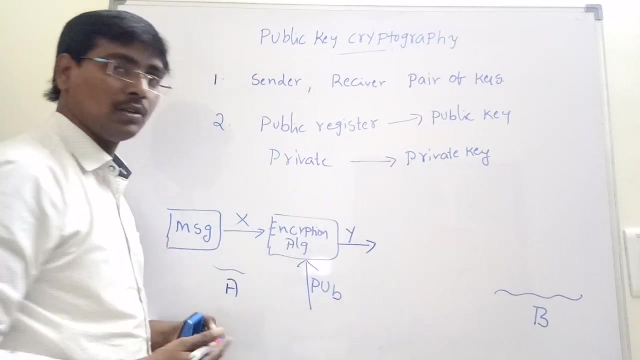 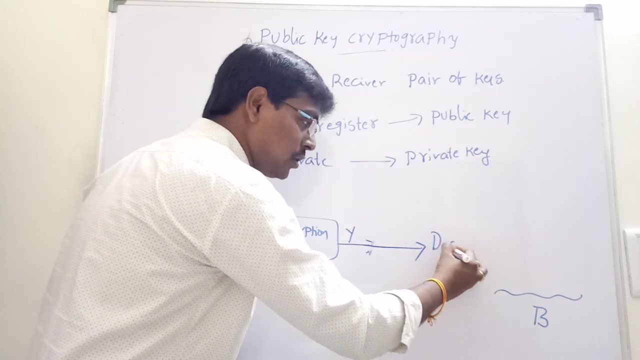 The first one is: user A performs encryption using public key of B, Because public key of each user is known by everyone After performing encryption. suppose, if the message is Y Now, this message is transferred to user B Decryption algorithm. 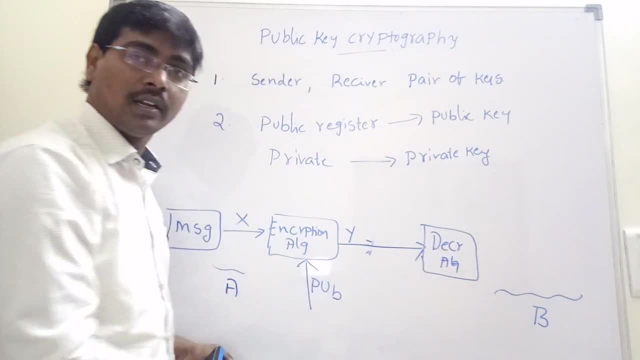 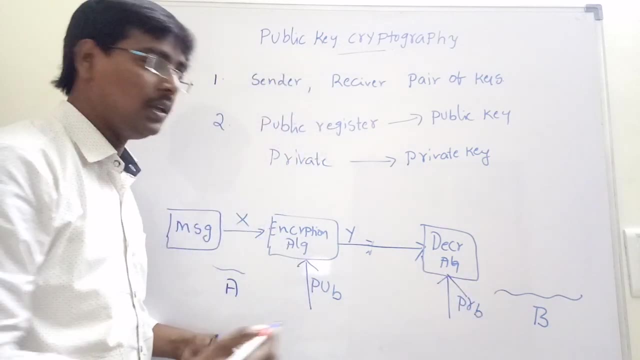 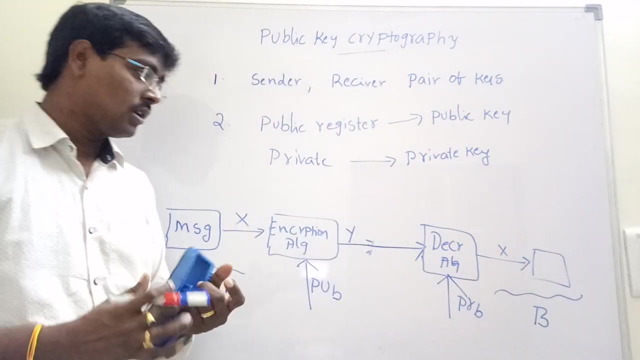 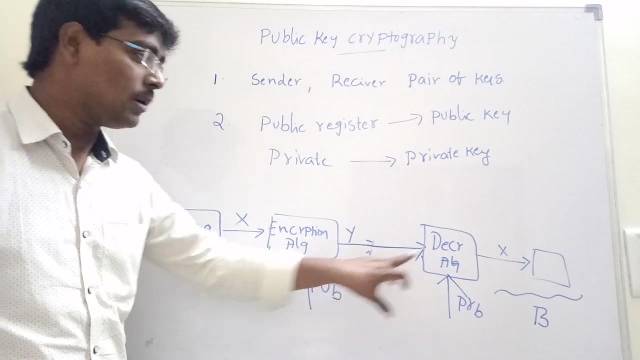 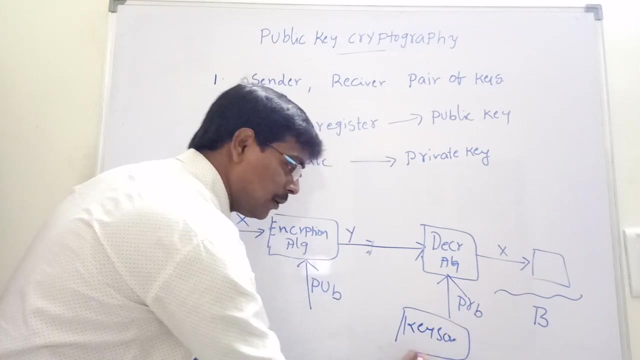 At decryption algorithm. at decryption algorithm we are providing decryption using private key of B And it produces the final text X. So I will explain the procedure Here in this example. first, the message is encrypted by using public key of B, For example. this is key source generator at B side. 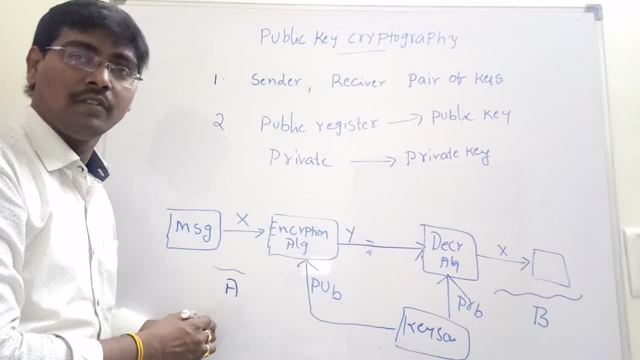 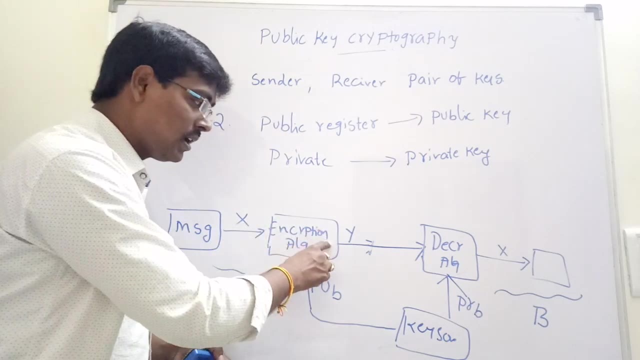 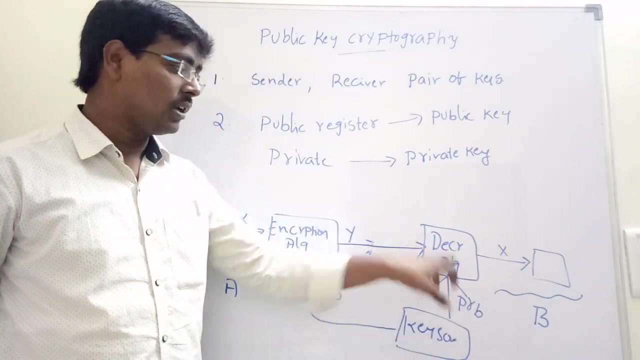 So the public key is visible to each and every user. So by using B public key, user A performs encryption. Now the encrypted message is transferred into receiver. Here B only knows the private key, That is, the Y, is received by many number of users. 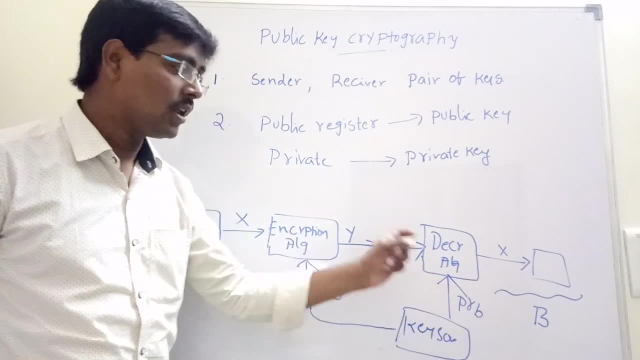 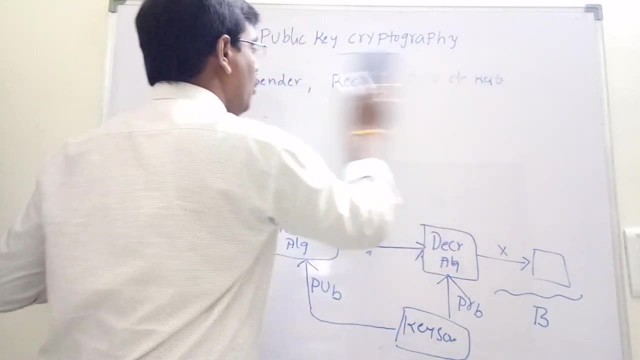 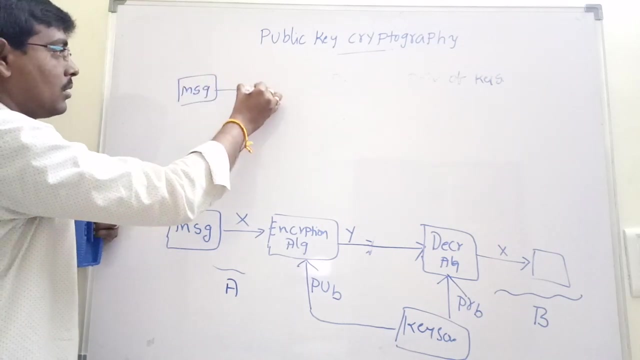 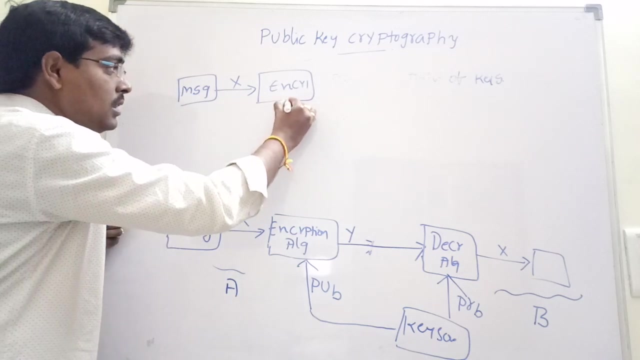 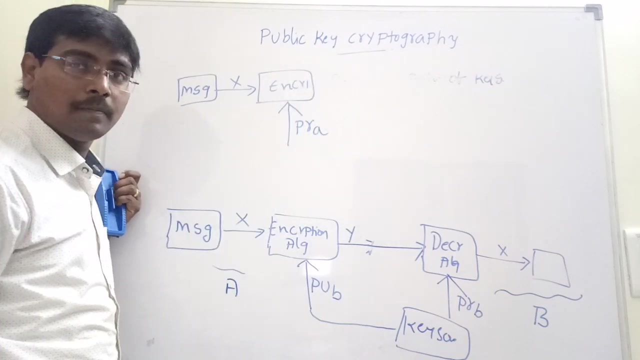 Only the actual recipient only decrypts the message Because PRB is the private key. In the similar fashion, we are moving to one more type of encryption. Suppose the message is encrypted by using some encryption algorithm In this step. suppose we are encrypted by using private key of A. 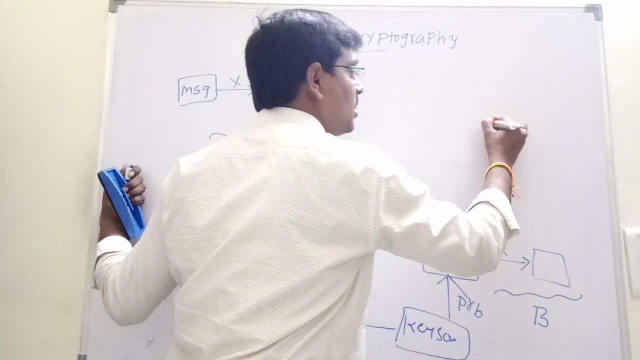 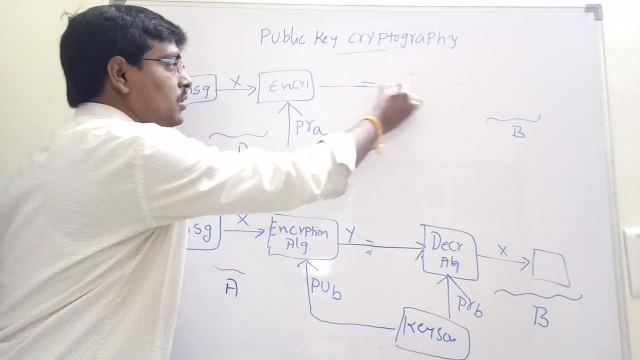 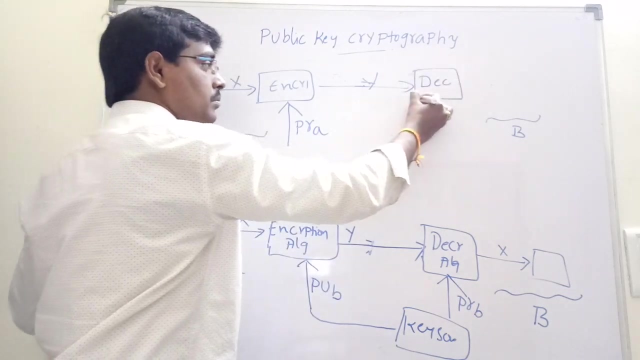 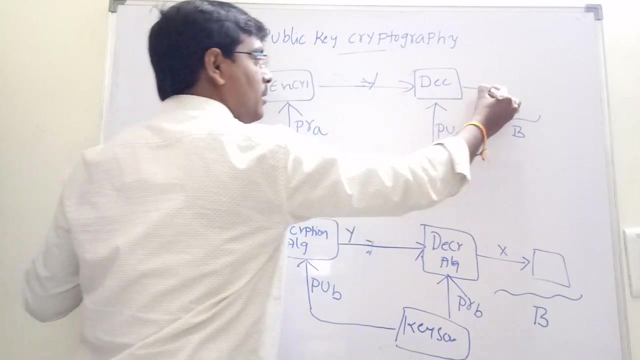 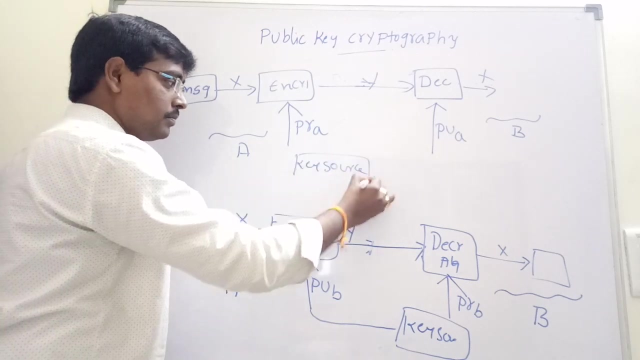 Here, source is A and destination is B. Encrypt the message using private key of A. Whenever we transfer the message, it decrypts the message by using public key of A, Suppose this is some key source at A side. So these are the two possibilities of encryption and decryption. 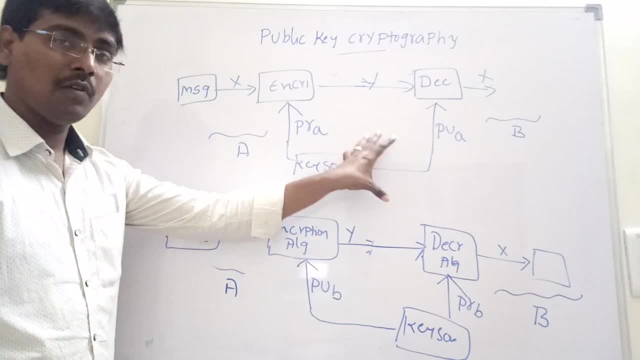 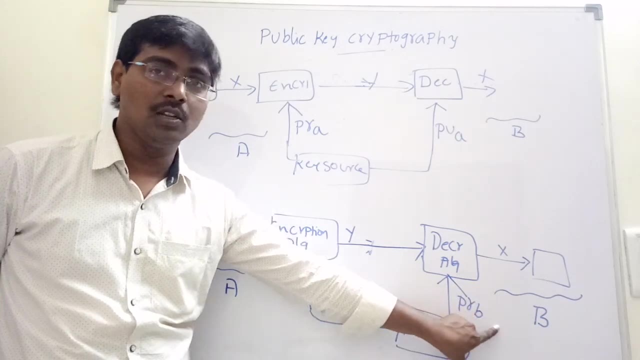 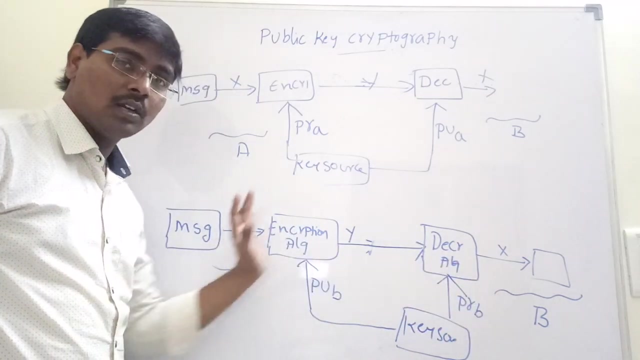 By observing these two figures, to perform both encryption and decryption we are using only one pair of keys of a single user. In this case we are using only user B's keys. Suppose user A wants to send some message to user B. 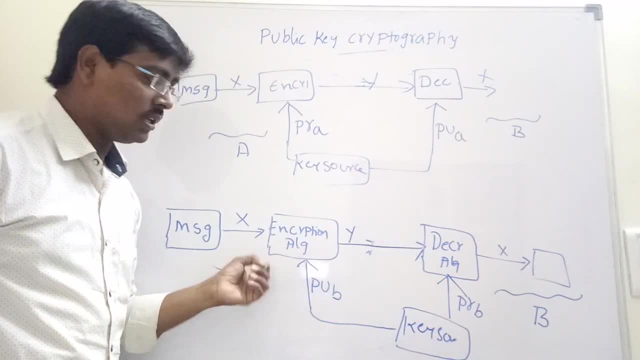 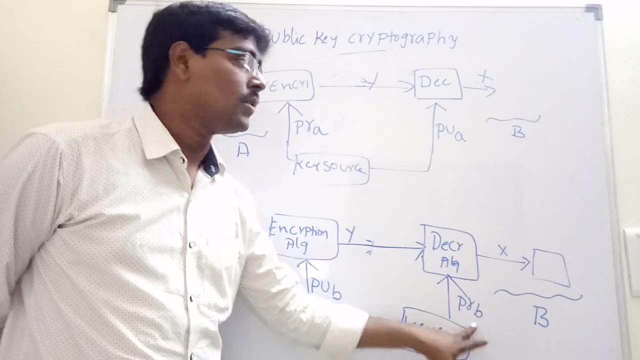 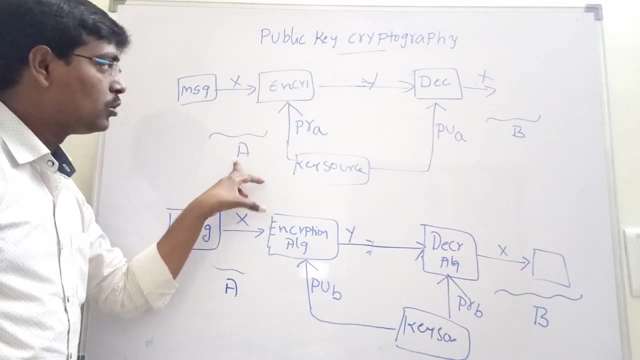 If we want to use user B keys at encryption, we are applying only public key. At decryption we are applying private key. Similarly, suppose user A wants to send some message to user B At encryption, user A applies his private key and performs encryption. 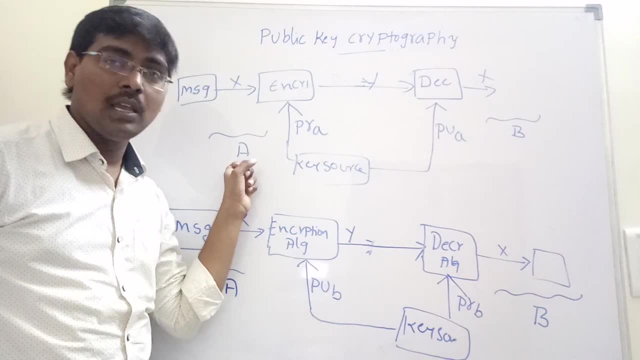 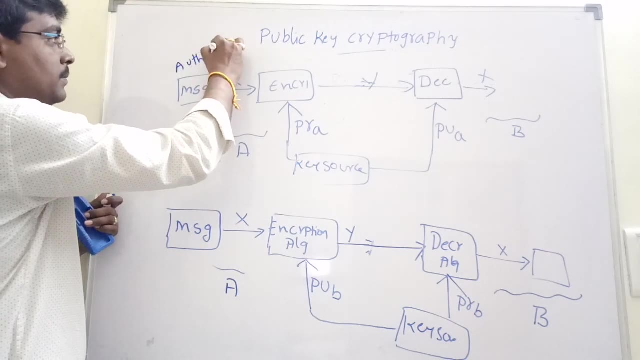 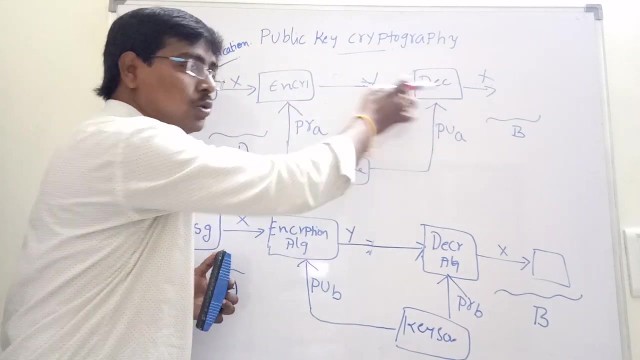 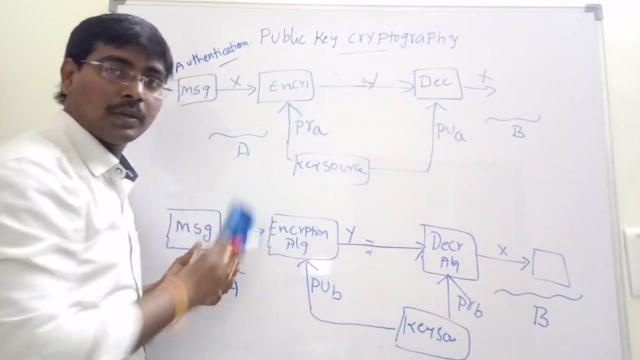 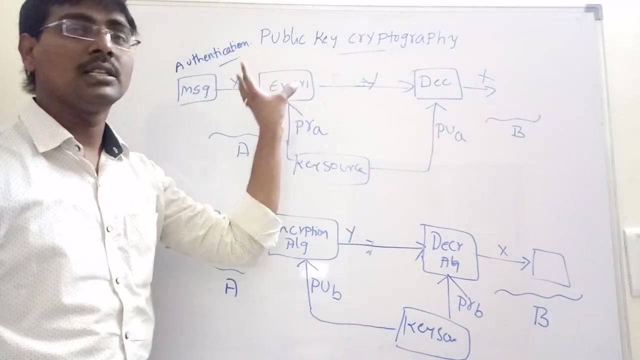 User B applies the public key of A to perform decryption. Simply, this procedure is called authentication. Authentication means simply, these two are corrupted. User A and user B are some connected, That is, one is authorized person of another. So here B only knows that the message is encrypted. 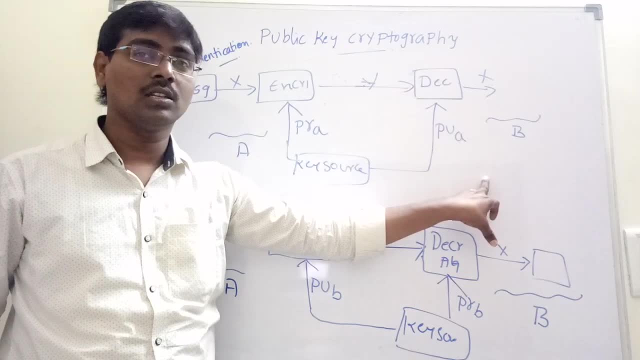 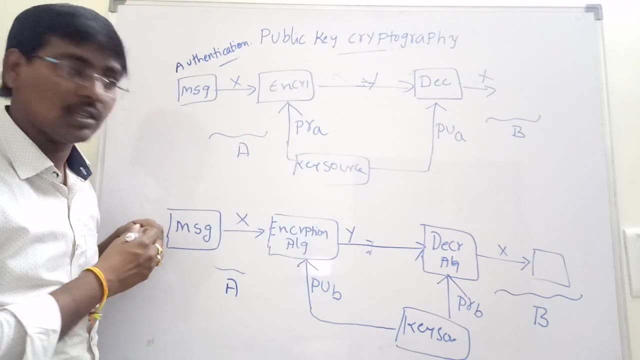 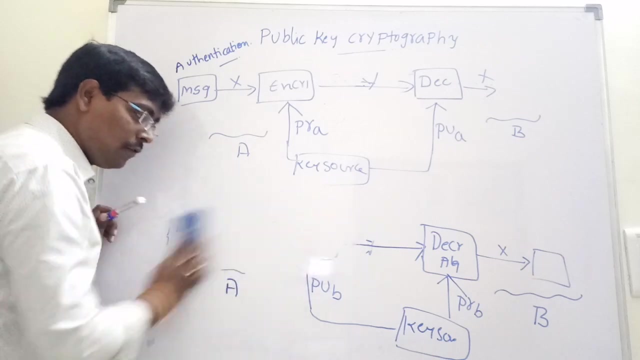 All other recipients, that is, all other users in the system, doesn't know whether the message is encrypted or not encrypted. These two are two types of encryptions. In both the cases, we are using only a single pair of keys. Suppose, if you want to perform confidentiality. 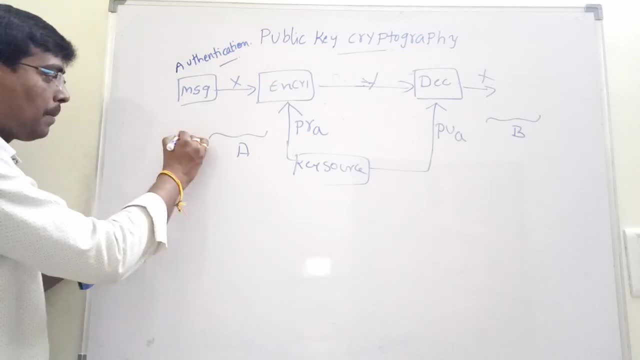 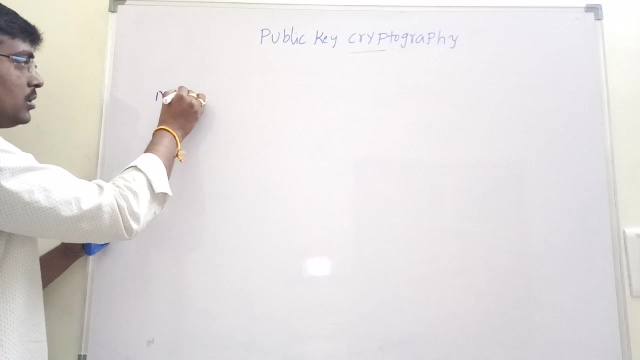 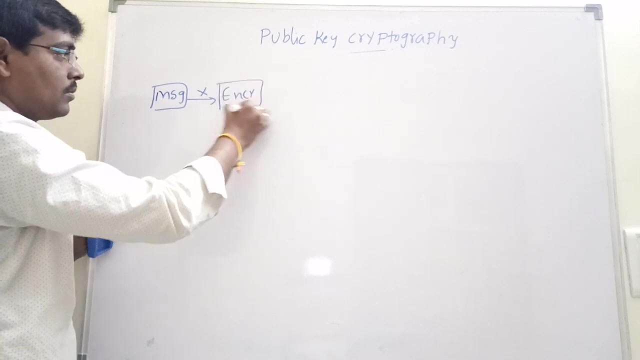 if you want to perform confidentiality, perform two encryptions at source side and two decryptions at destination side. So now we will discuss confidentiality. Suppose this is the message. The message X is: perform encryption Again. suppose it produces Y Again, perform encryption. 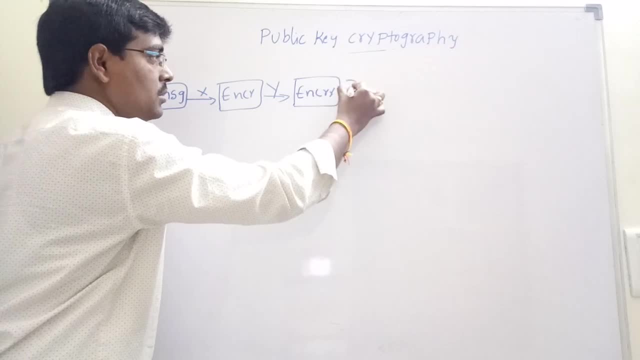 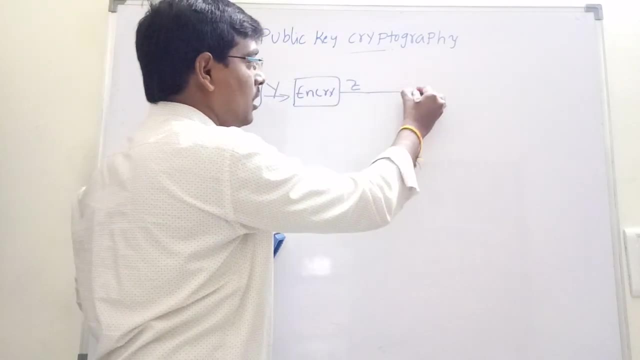 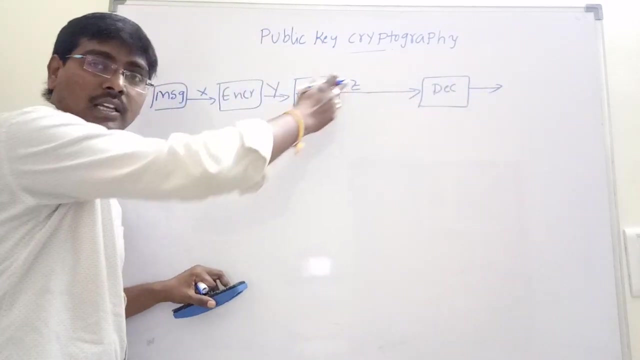 Suppose it produces message Z. After first performing encryption, it produces Y. After second performing it produces Z. Now the Z is transferred to the receiver. Suppose at the receiver: first decryption. first Z is decrypted. It converted into Y. Next Y is decrypted. 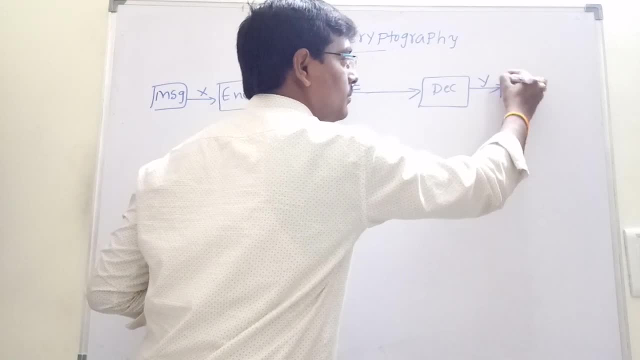 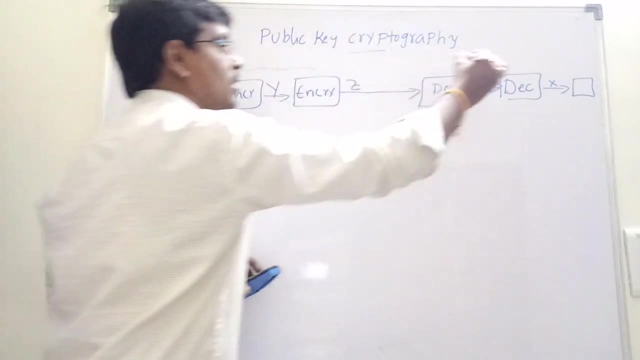 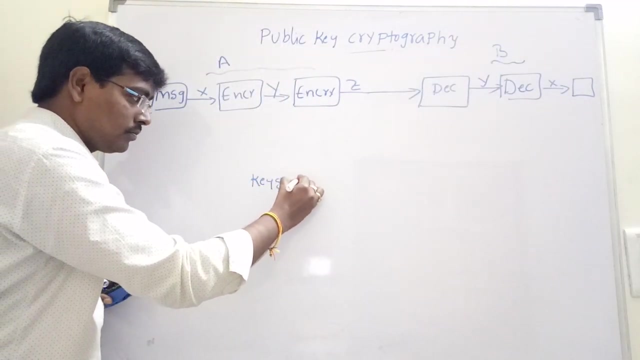 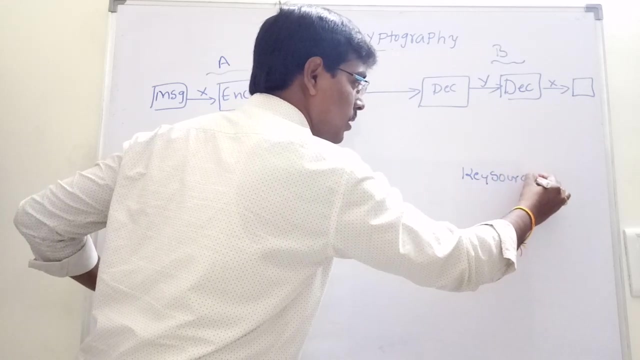 It converted into X, So we are receiving the message. For example, this is user A. This is user B, User A, user B. Key source at user A side. Key source at B side. Key source at user A side. and key source at B side. 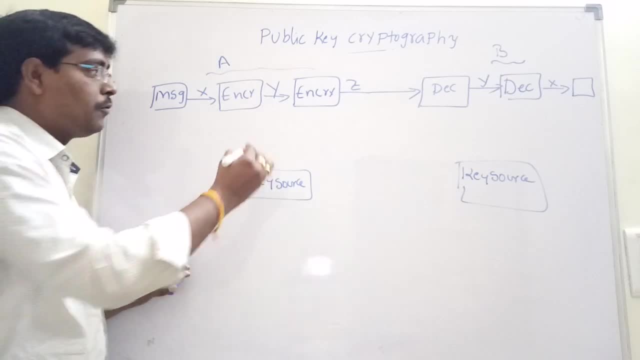 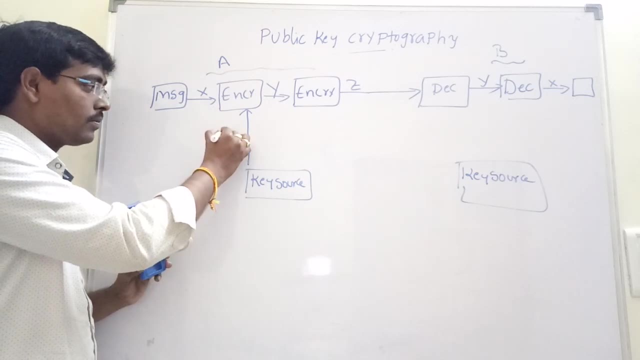 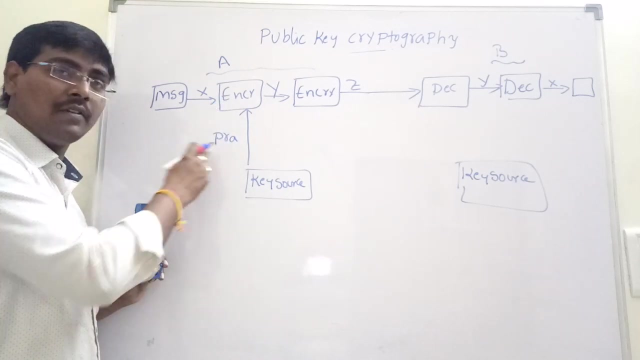 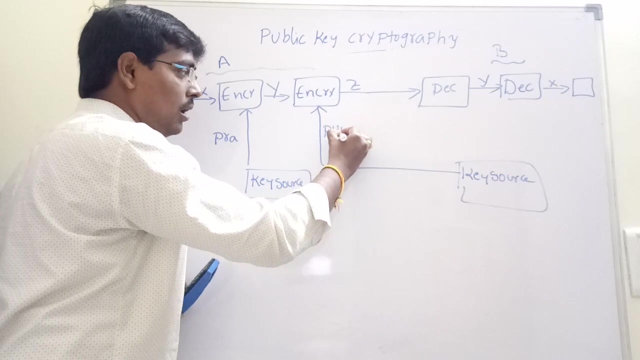 Suppose with the first two encryption: if you are encrypted, suppose, by using private key of A, Suppose with the first two encryption. if you are encrypt the message using private key of A and its second encryption, we are using public key of B. 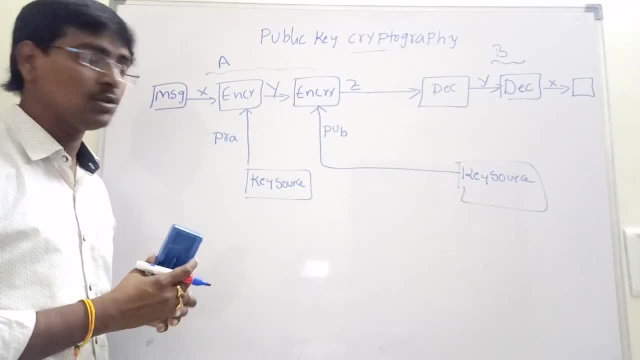 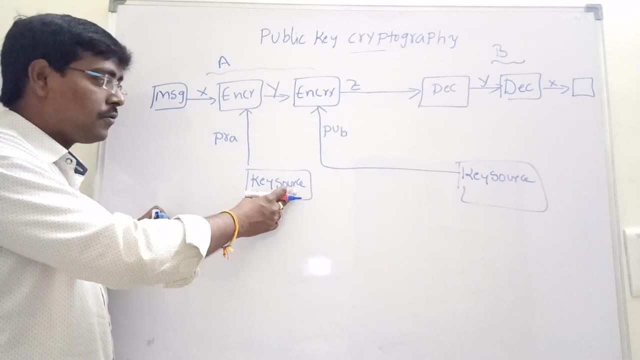 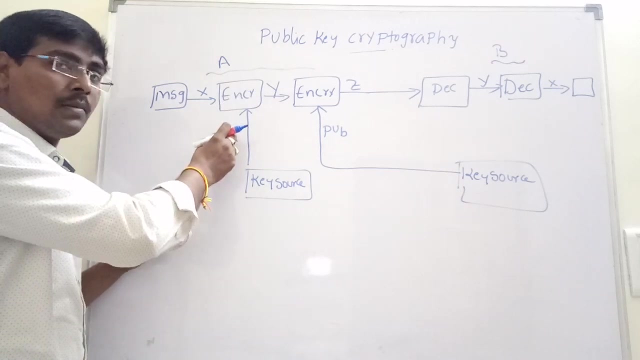 That is simply, I am combining the previous two approaches: Key source of A, key source of B. It will generate PRA- private key of A- and PUA- public key of A. Similarly PUB and PRB. First to encrypt the message using private key of A. 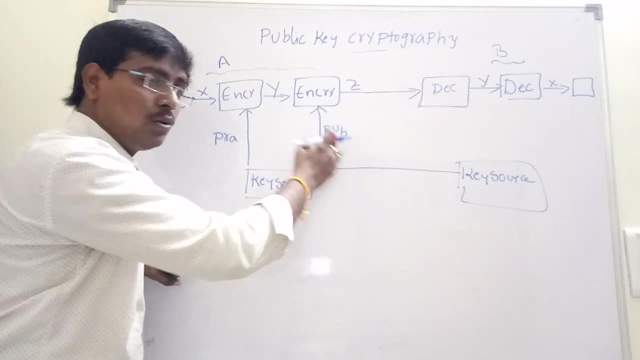 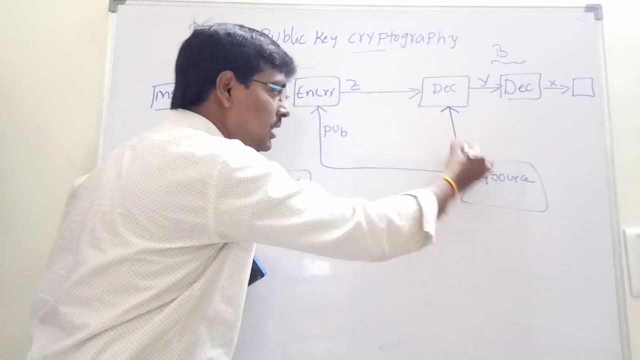 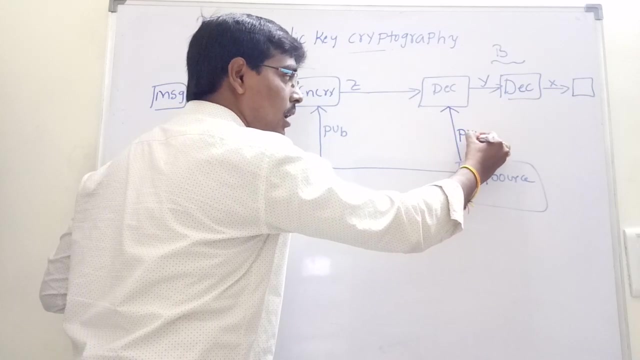 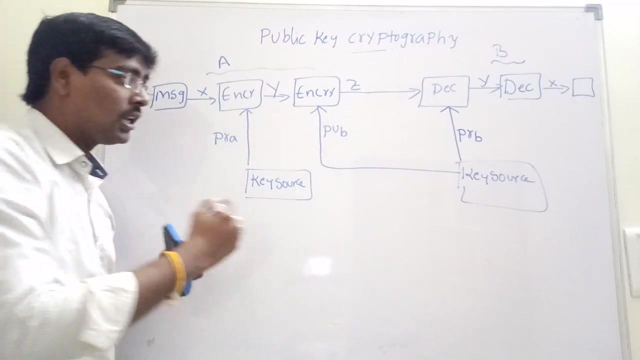 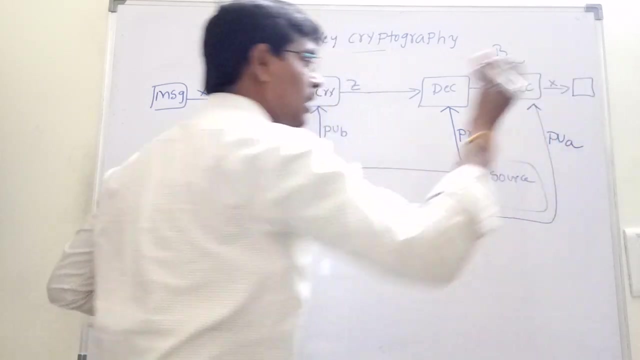 And the encrypted message is again encrypted using public key of B. It produces Z. Now this Z is decrypted. This Z is decrypted by using private key of B, By using private key of B, And this one is decrypted by public key of A.